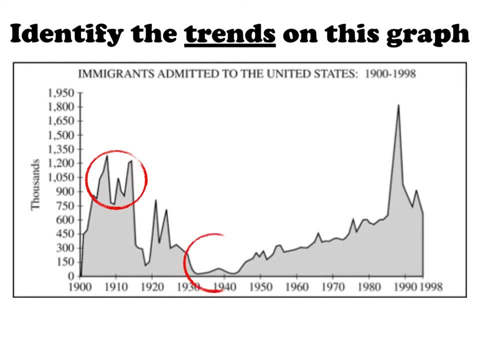 So we see a graph here. So we see a pretty large spike in immigration there. Then we see a huge decrease or trough in immigration and we can attribute that to immigration, anti-immigrant policies that were passed in the 1920s in combination with the Great Depression and World War II. 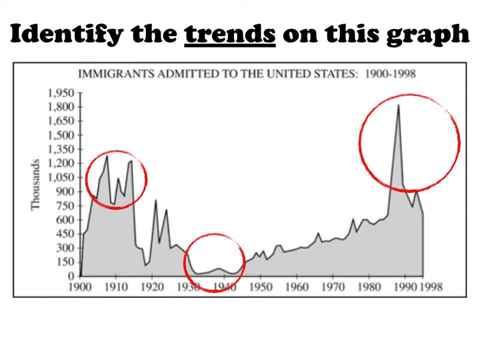 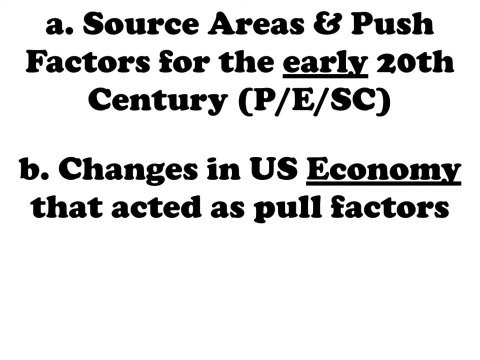 Finally, we see another huge spike here in the 1980s, 1990s at that time. So those are the major trends that we can see in this graph and these are important to understand in terms of answering this question. So the first part of this question is identify the source areas and push factors for the early 20th century immigration. 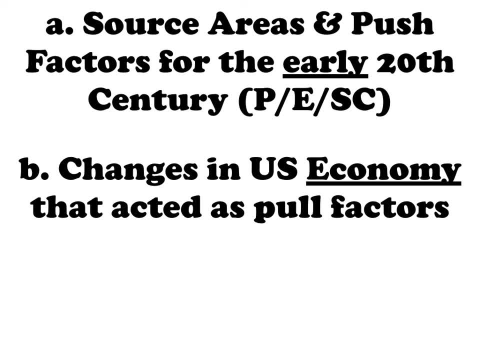 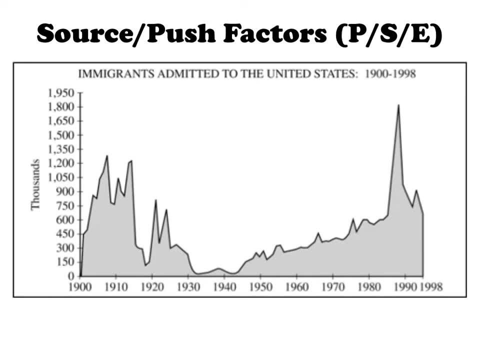 political, economic and sociocultural, as well as changes in the US economy that acted as pull factors for this immigration wave. So we are dealing specifically and we're targeting this immigration wave, which is the beginning of the 20th century. 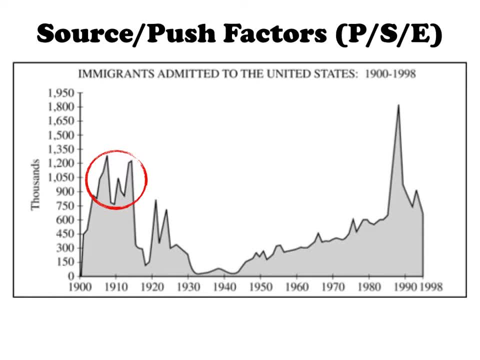 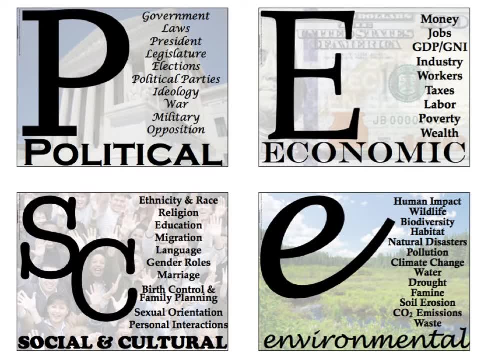 It's very important that we don't get confused between the two separate immigration waves. So with this immigration wave we're going to look at political, economic and sociocultural factors. This is a reminder. political factors are things that have to do with government laws, presidents, legislatures, elections, ideology, war, military opposition to the government, etc. 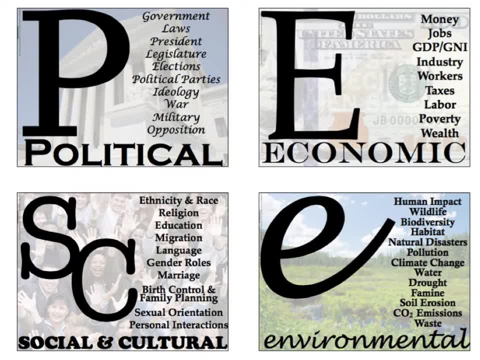 Economic factors are anything to do with money, jobs, employment, industry, workers, poverty, etc. Social and cultural factors are things that have to do with ethnicity, race, religion, Education, migration, language, gender roles, etc. For this topic, we are not going to go into environmental factors, although oftentimes environmental factors can be a push factor in terms of immigration. 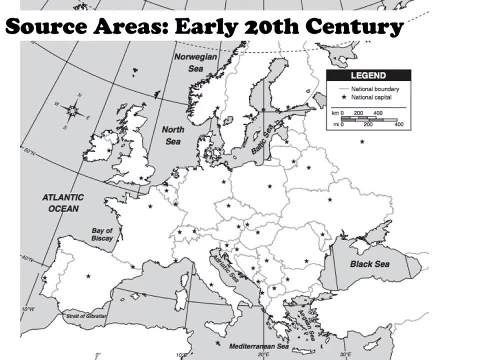 So for the early 20th century, the source areas were predominantly in Europe. In terms of pure numbers of immigrants, the vast majority were coming from Europe And specifically they were coming from two regions in Europe. They were coming from Southern Europe. 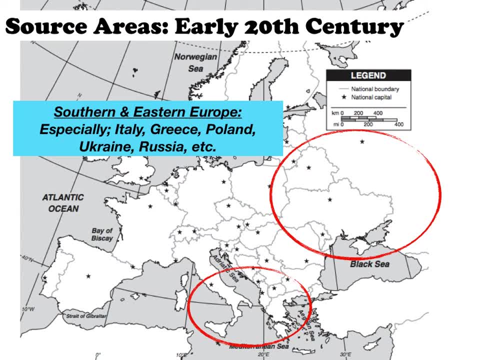 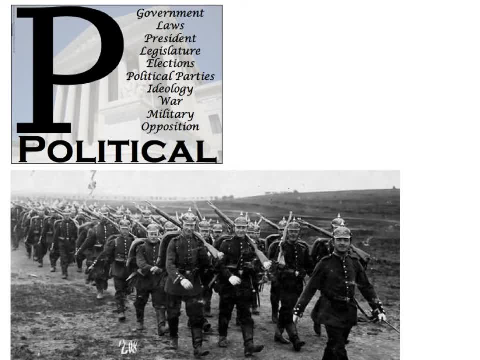 But in terms of numbers these are the major areas. Now we're going to look at push factors. So what was going on in these areas at this time to force people to leave their homes? So one big push factor at this time was war. 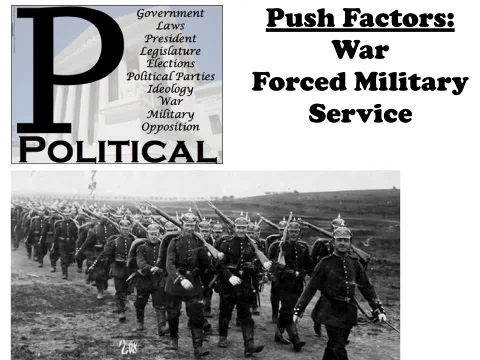 Not just World War I, but also other small regional wars that had occurred prior to, And not just World War I, but also other small regional wars that had occurred prior to, And not just World War I, but also other small regional wars that had occurred prior to. 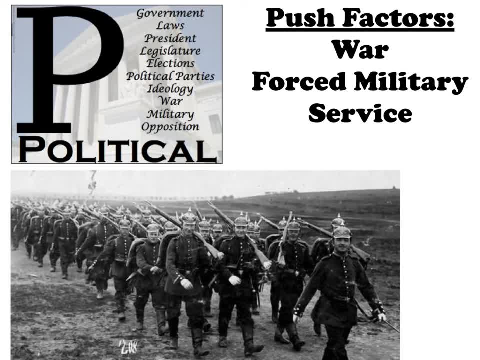 And not just World War I but also other small regional wars that had occurred prior to. So the first two had pushed countries and empires to create forced military service. So even in times of peace people were forced to serve in the military. 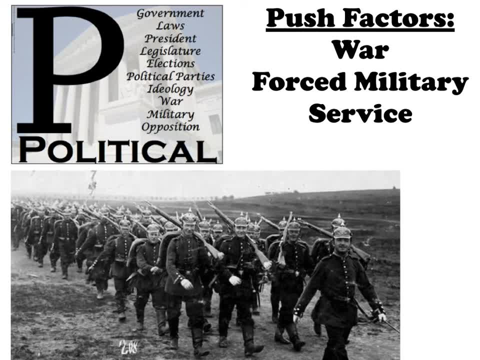 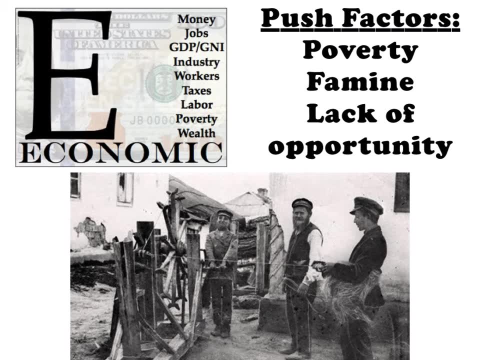 Many people didn't like this and they wanted to leave for that reason. Other major push factors were economic. At this time in Europe there was a lot of poverty. This poverty led to famine. It also led to a lack of opportunity. People didn't necessarily see a future for themselves, living especially in rural places. 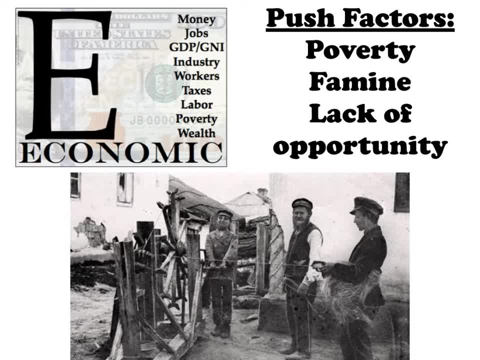 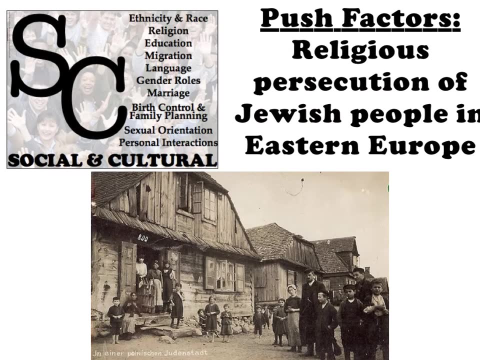 And so they saw the promise of employment and steady work in the United States as being enough to get them to get up and leave their homes and try something new. Finally, we have social and cultural factors, And the major push factor here was religious persecution of Jewish people in Eastern Europe. 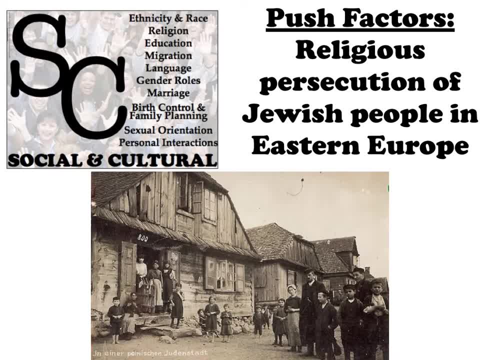 So Jewish people had been experiencing persecution for many hundreds of years. This is not the same as the Holocaust. Very important to understand. the Holocaust comes much later. Holocaust happens in the 1930s and 1940s, when there was little to no immigration from Eastern Europe to the United States. 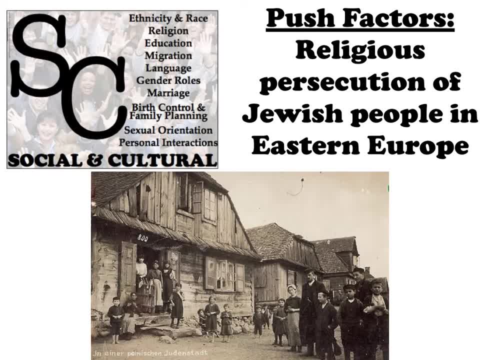 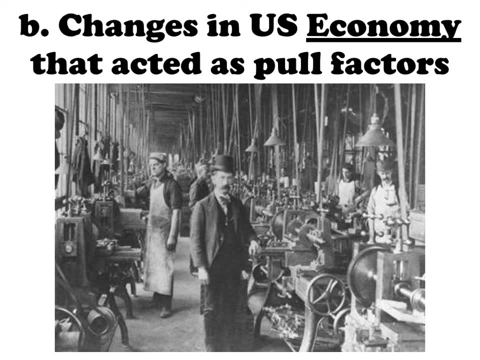 So this is pre-Holocaust, And there were things like attacks on Jewish villages, which are called pogroms, and other forms of persecution, So a lot of Jewish people fled at this time due to this. Now, the changes that were happening in the US economy were that the United States had undergone industrialization. 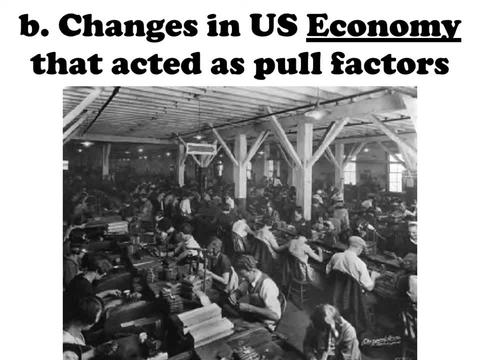 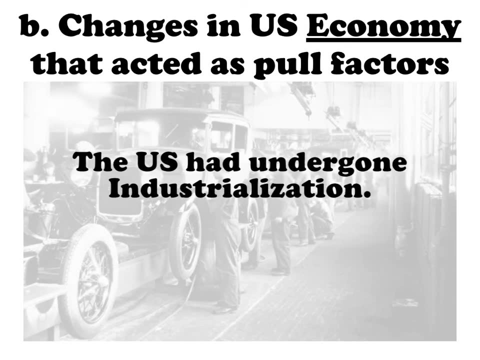 And there were many, many new businesses and factories opening. Much of the work in the US was still being done by hand, And so we needed people to fill these factories, So there was a huge demand for laborers. So, to summarize, the US had already undergone industrialization. 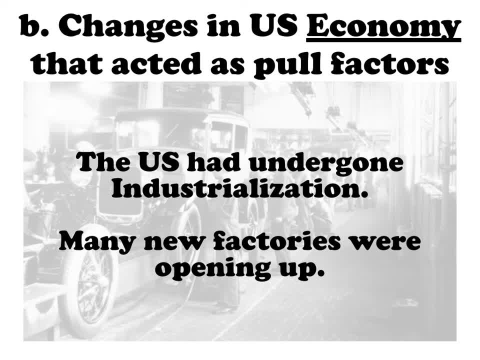 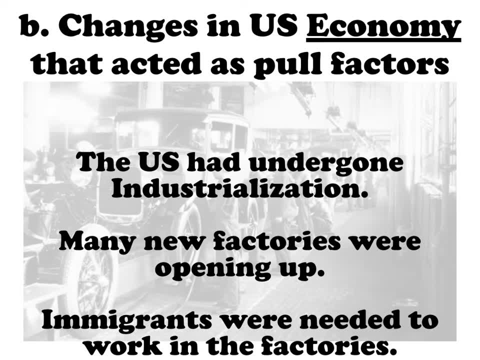 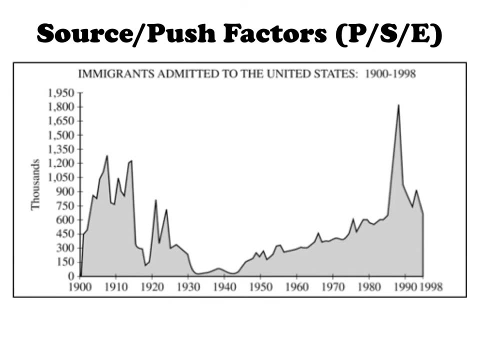 Many new factories were opening up And immigrants were needed to work in these factories. So these are all pull factors that contributed to this major migration wave in the early 20th century. So, going on to the second part of this question, it's examining the major migration wave that happened in the later part of the 20th century, in the 1980s and 1990s. 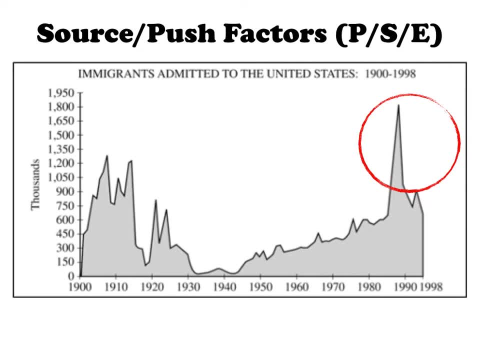 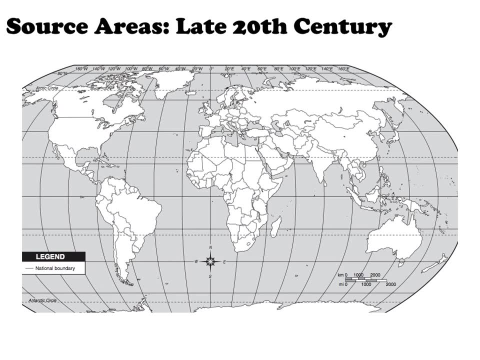 So first we're going to look for source and push factors And then we're going to look at changes in the US economy that acted as pull factors. So the source areas for this migration wave are quite different than in the early 20th century. 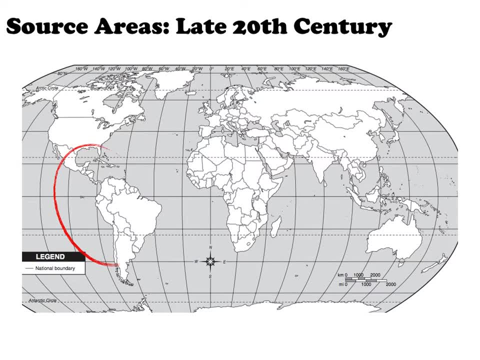 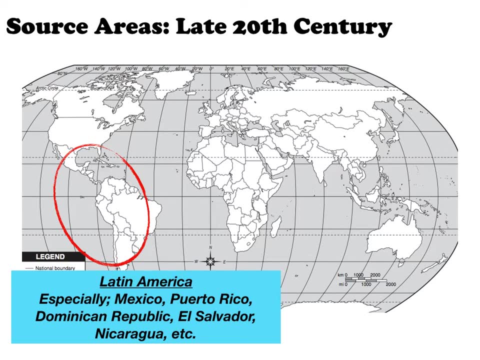 For the late 20th century, the US economy was very different. We're looking at two major regions, the first of which is Latin America, especially specifically Mexico, Puerto Rico, Dominican Republic, El Salvador, Nicaragua. These are countries with major amounts of immigrants coming in the 1980s and 1990s. 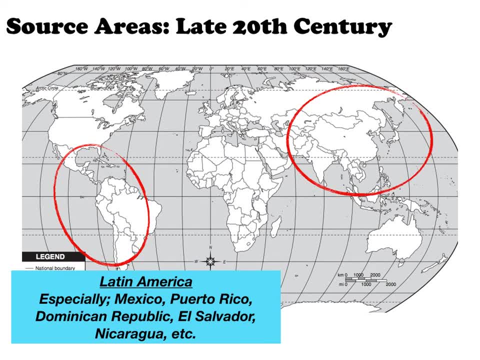 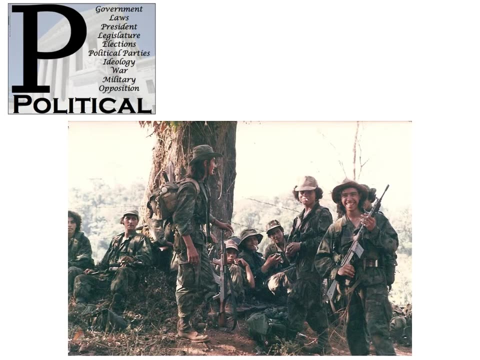 The second region that we're going to look at is Asia, So especially the countries of China, Vietnam, Korea and the Philippines. These are major contributors to migration in the United States in the 1990s. So we'll look at push factors first. 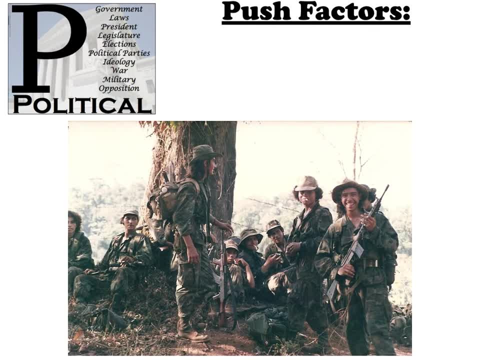 The first push factors that we're going to look at are political. At this time in the 1980s, especially in Central America, there were many civil wars going on, Again, forced military service, as well as a lot of guerrilla groups who also forced people into military service. 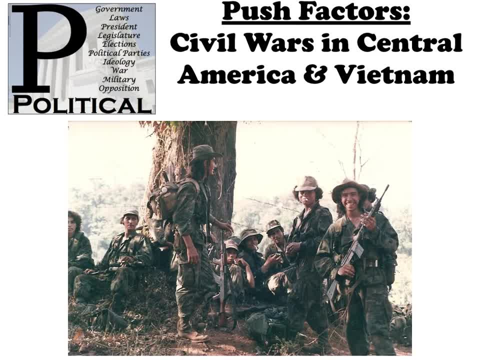 And a lot of people didn't want to participate in the wars or found themselves being on the receiving end of violence. So that really pushed a lot of people into military service. In addition, the Civil War or Vietnam War that happened in the 1960s and 70s and then the end result of that also pushed a lot of people out. 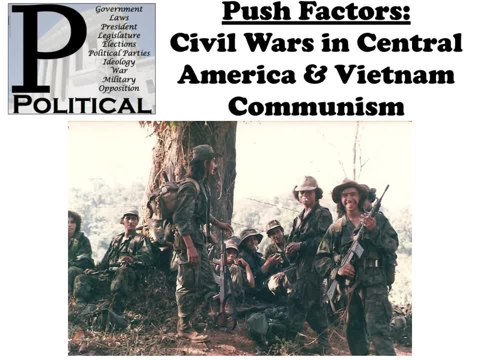 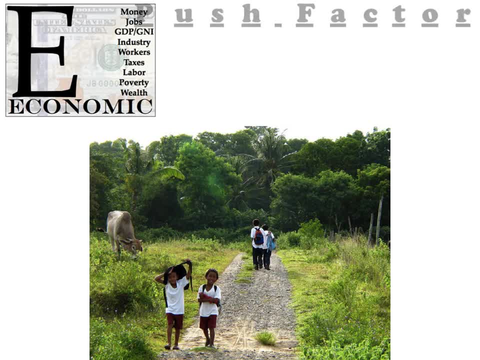 Finally, there was a flee from communism from Southeast Asia, including Vietnam, as well as from China. The next set of push factors that we're going to look at are economic. So the major push factor at this time, with this immigration wave, would have been poverty.